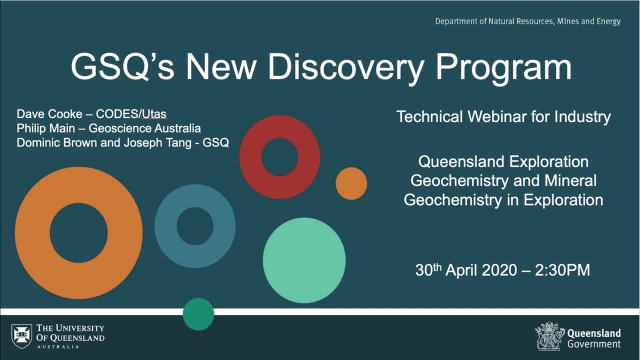 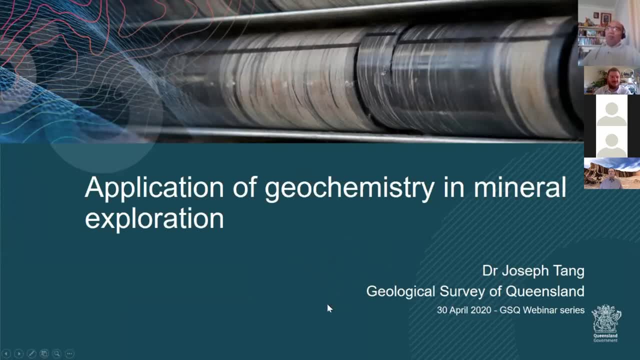 In this presentation today, I'm going to talk about the application of geochemistry in mineral exploration. Basically, what I'm going to do here is to highlight, you know, the exploration within Queensland itself and to talk about the different data sets. you know, that's. 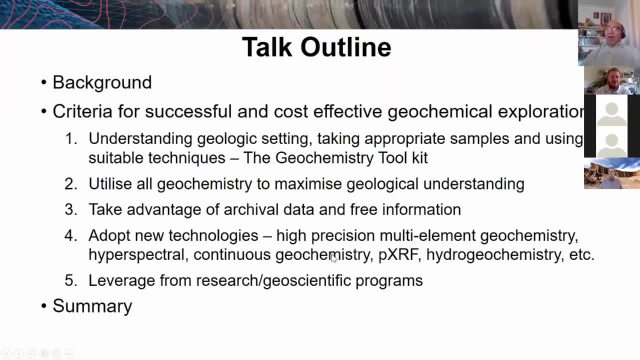 available to help industry. In this talk I'm going to talk about the background of exploration, geochemistry, basically about the transformation of chemistry. you know from. you know what it was until what it's going to be, Then I'll sort of delve into. 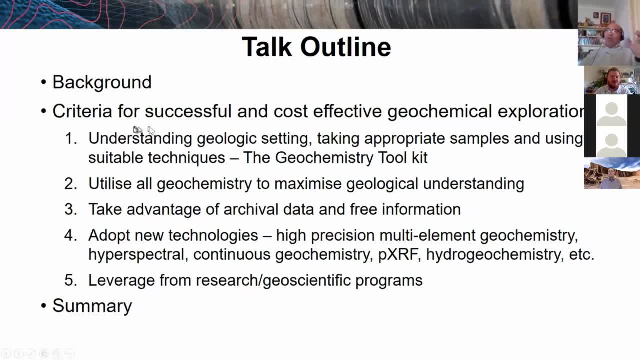 the core of this talk to sort of discuss the different criteria for successful and cost effective, you know, exploration, basically understanding the geological setting so that we could find the right samples, the right techniques- which is basically what the geochemical toolkit is- And then highlight the different data types. that's available. 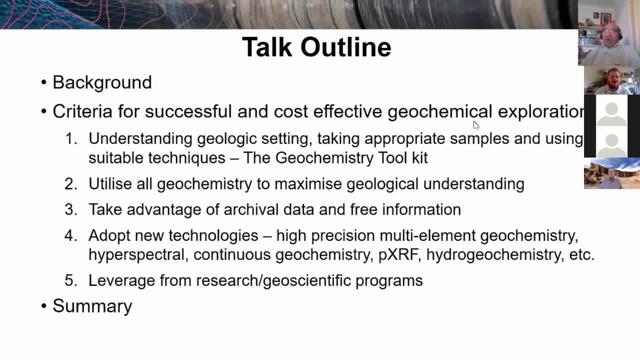 In Queensland and the importance of utilizing, you know, all the different data, including the majors and trace elements, to get a good geological understanding to be effective in this geochemical exploration. Also, it's really important to take advantage of all the archival data and a free knowledge base information that GSTO has produced as well. 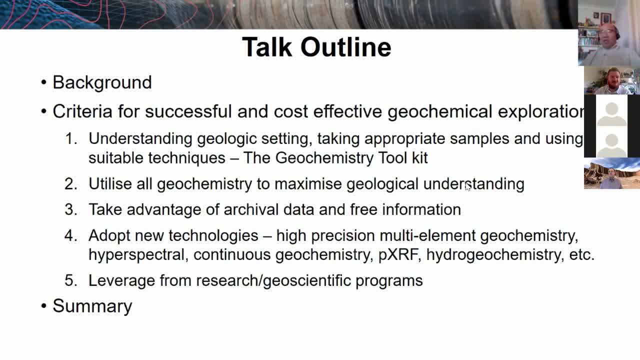 as the collaboration that we have done with other organizations so that this could be used by industry To sort of expedite as well as to expand the asset of, you know, exploration targeting, And it's really important. I think you know we have come to a phase where most discoverable 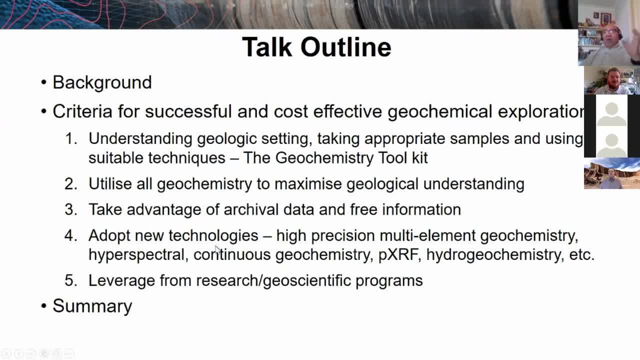 you know, deposit has been found. And then we have to adopt new technologies like high precision, multi-element geochemistry, hyperspectral, continuous- you know- XRF scanning, et cetera, to help with the future discovery. And finally, I'll discuss about the leverage with research. 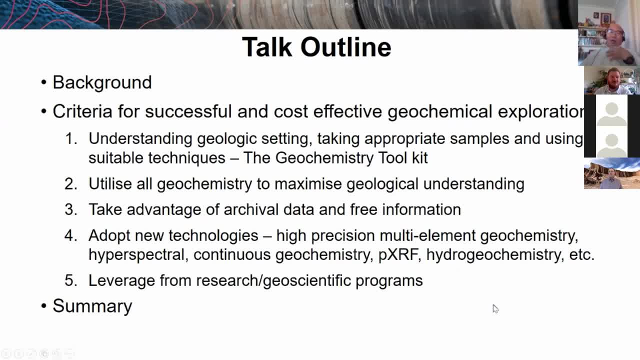 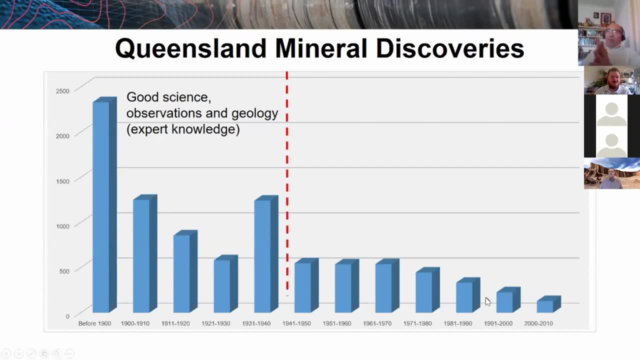 organization and other geoscientific programs you know, to enable this sort of, you know, work to progress, you know, at a minimum risk or exploration risk to the company itself. The first pictures you know shows here shows the mineral discovery in Queensland. 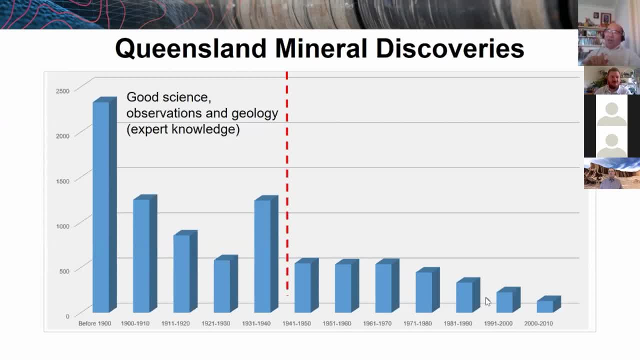 Basically, Queensland has been a very active exploration target, you know, for the last 150 years Before the Second World War. within this first 80 years or so, a lot of this discovery were done just based on good science, good geology and good knowledge base, which we brought in miners from overseas as well as. 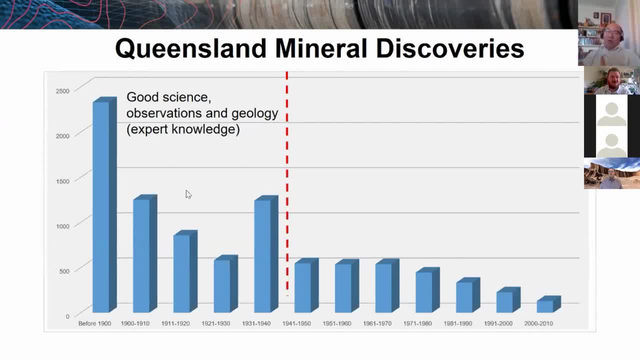 from other parts of the world to find the gold and tin deposits you know, in both Palmer River and in the Darling Downs. It's only after the Second World War. you know the geochemistry, geophysics and you know geological modeling were used in the discovery of mineral. 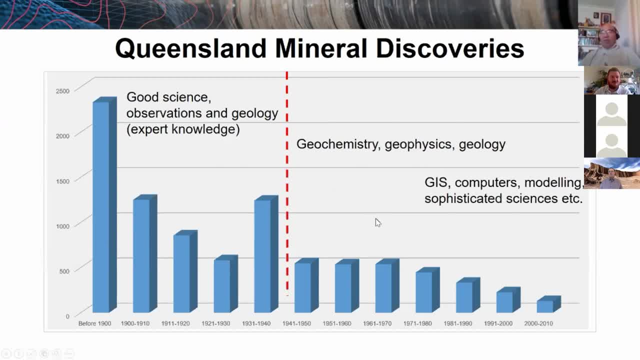 deposits. And in the 80s, where computer becomes fashionable, things like GIS, you know, modeling and other sort of computer-related science were adopted. Nonetheless, if you look at the train of, you know, discovery, it starts to sort of fall off And we were sort of held back, you know. 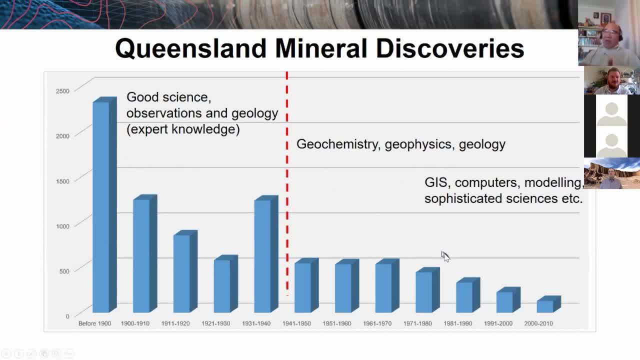 by good science, you know, until about 1980s, And after that it starts to taper, And one of these reasons is that a lot of this easily discoverable deposit has been found And then we are forced, Or we have to face the highly difficult to find, you know, deposits undercover itself. 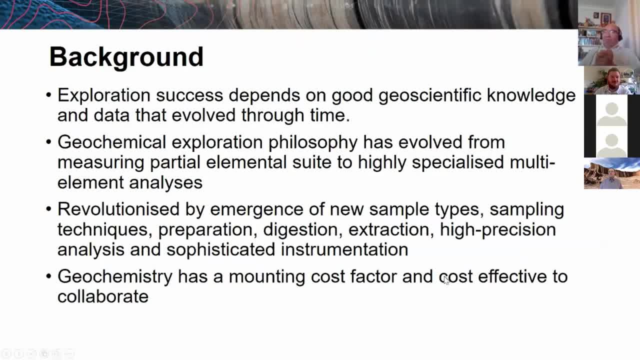 Well, the background of geochemistry, or the success of geochemistry, depends really very much on good science, that's, good knowledge base and as well as good data, And both science and data evolve through time, And that's a really important sort of concept, I think. 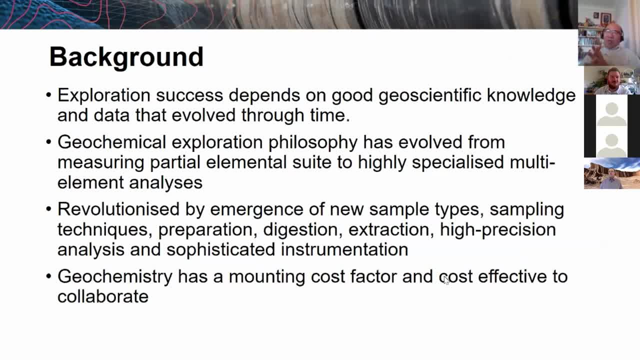 for explorers to understand. In terms of geochemical exploration, The philosophy has changed tremendously in the last 50 years. In the early part of these 50 years, most geochemistry are there to actually identify or to analyze material, which one needs to know what the content is to decide whether it's an ore material or it's not. 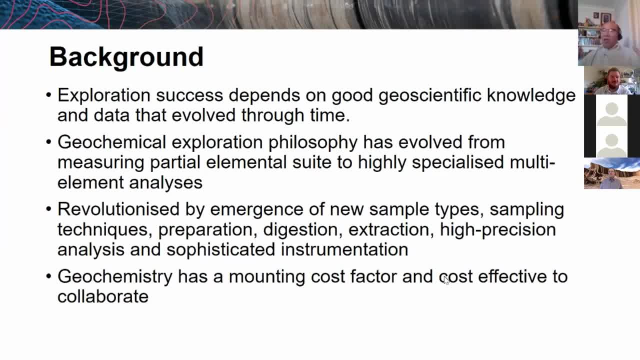 And then to look at the expansion of those non-ore materials outwards, to basically define, in a way, the margins of this ore deposit is, Whereas later on, geochemistry, exploration geochemistry- has moved into detection work where it has, you know, used very highly sophisticated multi-element chemistry as a tool to try and 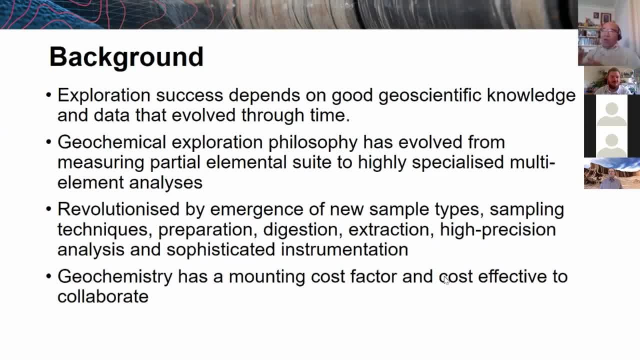 sort of discover the pathway of chemistry to where site is. In other words, it's used as a tool to try and sort of decide or discover where the source region is. So that's the big sort of shift, The shift from the determinative, you know, sort of chemistry to detective chemistry. 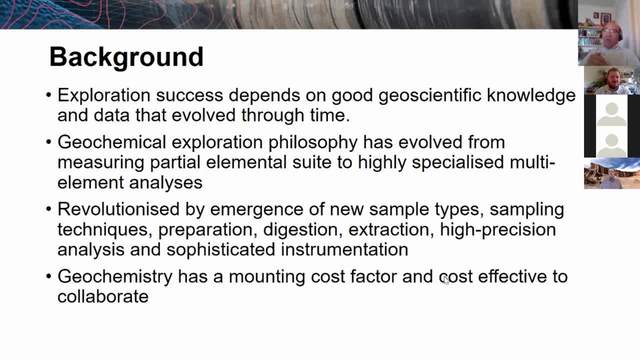 With this revolution there is a lot of emergence of new exploration science And basically it talks about, you know, new samples, new sampling techniques, preparation, digestion, extraction techniques, that's you know, new And also very sophisticated instrument that 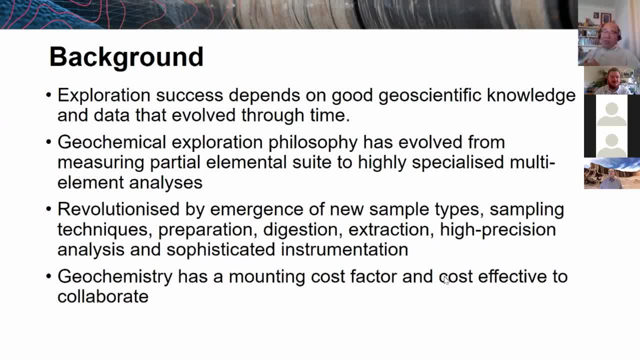 enables, you know, the industry to find very high precision analysis itself. Well, with all these advances in chemistry, exploration becomes very expensive, And it's generally in today's you know sort of exploration. it's balancing between cost factors and how. 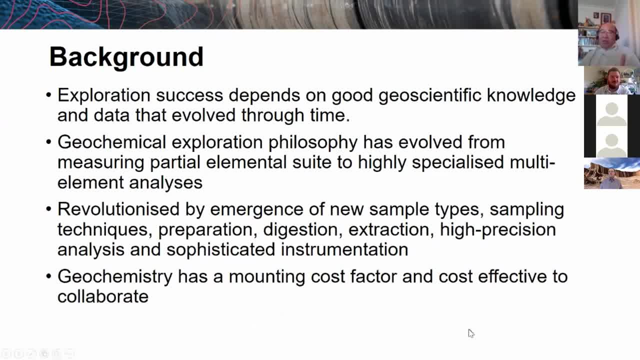 effective it is And that's why I will talk about collaboration and, you know, archival data sets. you know, in the later part of this talk, where you could cut down some of these costs by using ideas and you know sort of finding that has been, you know, made. 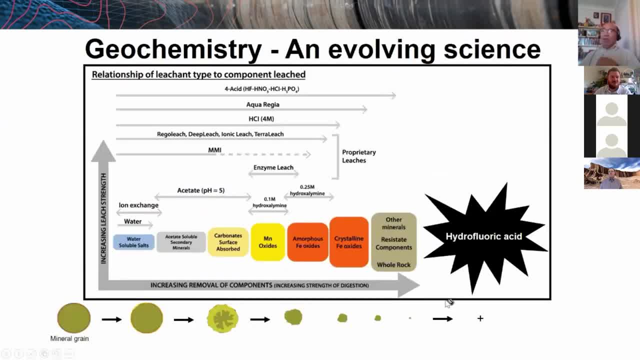 by scientific organizations. This is how the chemistry has evolved over time. It is an evolving chemistry, As I mentioned in the earlier part of the century. most of these geochemistry is within this rim. where you- this is the concept- is when you have a grain, a mineral grain. 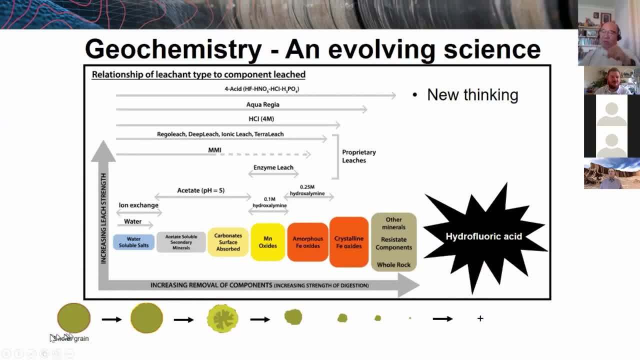 and it has a sort of thin coating of transcend mineral mineralization on top or just mineral on top of it In the earlier years a lot of this conventional chemistry, because a lot of these mineral grains are derived from all material itself. So to determine how good that all material is, 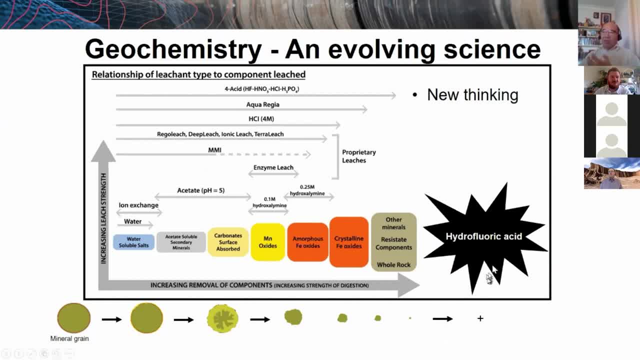 you try and dissolve all of them as complete as possible, And so it come up with this multitude numbers of acids, from the highly corrosive hydrofluoric acid that digests everything, to the four acids, to the aquaviridia and to the different acids. 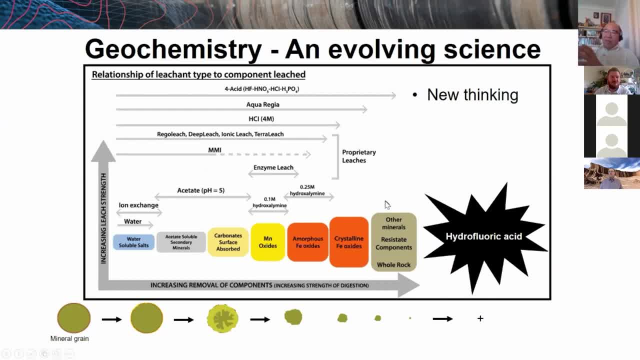 pure acids of different concentration. The idea is to get them as close as possible, a chemistry that reflects the ozone or the material that you collect, so that you know whether it's all or it's not. However, with the change in the philosophy, where a lot of these deposits are undercover, 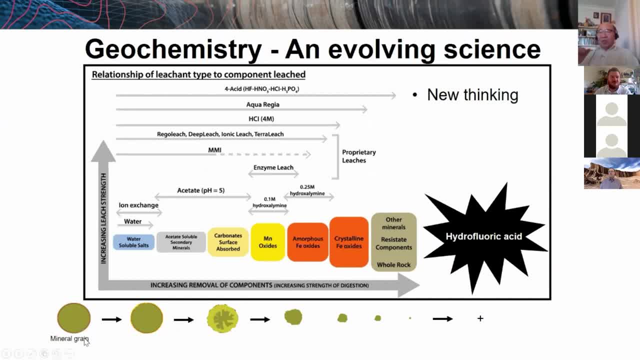 a lot of this chemistry, the transient chemistry, goes through substrates or discover sequences that has nothing to do with the mineralization and a lot of this chemistry is sediment substrate that you don't want the chemistry. for example, if you were to dissolve everything, you get a very strong dilution factor from that chemistry, from. 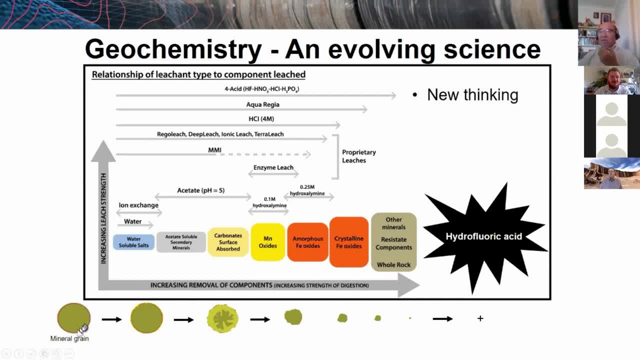 the mineral grain. what you are interested is just that little veneer of chemistry on the grain itself. and so it came out with a whole series of partial digestions, because for the more aggressive ones that digest you know more into the grain. to ones that just edge or just displace, those you 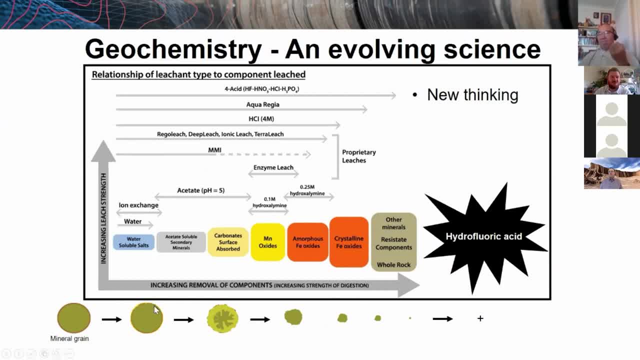 know, exchange cation, you know, within the material itself. and so this is where this big shift in term expression, geochemistry is, and i think you know explorer has to recognize that big shift from a determined native chemistry into a detective style chemistry to try and sort of. 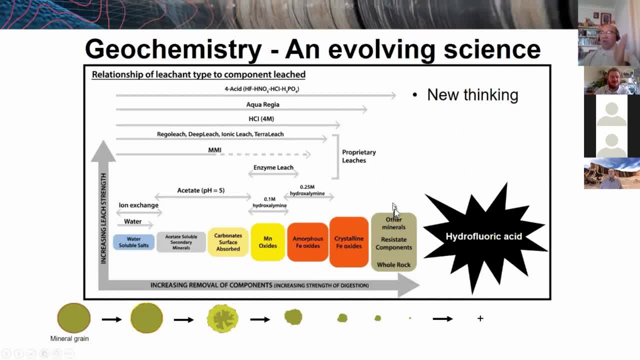 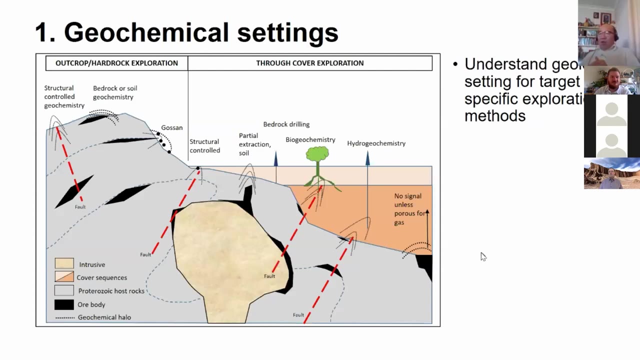 discover where the new deposit is. therefore, the geochemistry expression has evolved tremendously, with a lot of new thinking, a lot of new technology, and therefore it requires a lot of new equipment or instrumentation to achieve that. now, what? what's the sort of you know requirement for a successful geochemical exploration program? basically, i'll go into the 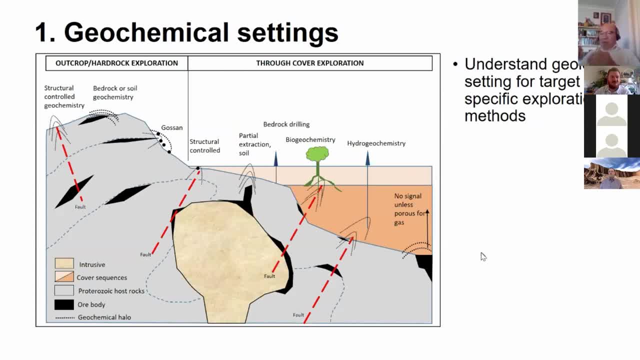 five points that i mentioned earlier. the first of the um, the um criteria, is to be able to understand the geochemical setting. basically, there, in geochemical exploration, there are only two settings: the outcropping and the undercover setting. both of them had very similar geochemical 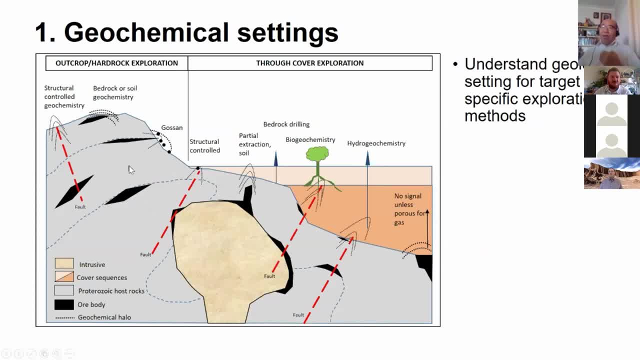 sort of you know um expression, except one of them is undercover. the difference of them is: is um? i'll just go through them briefly. a first scenario in the explore, uh, exposed- area is that the actual ore material gets exposed to the surface and therefore when you pick a surface in a sample, just analyzing it just, 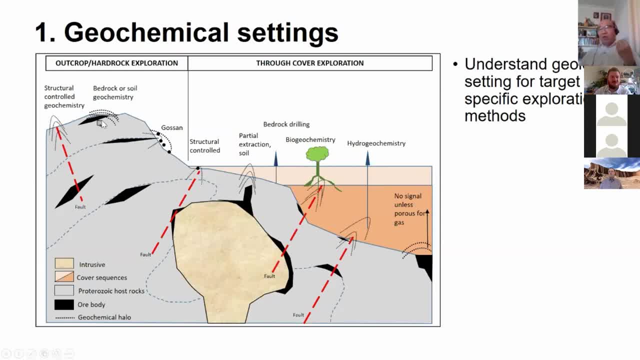 dissolving the whole thing, you will have a good idea what's the grade of you know of that ore material is. the second sort of you know scenario is when the material gets to the surface and it's it gets broken down into daughter products like gossens, laterite etc. and by analyzing those 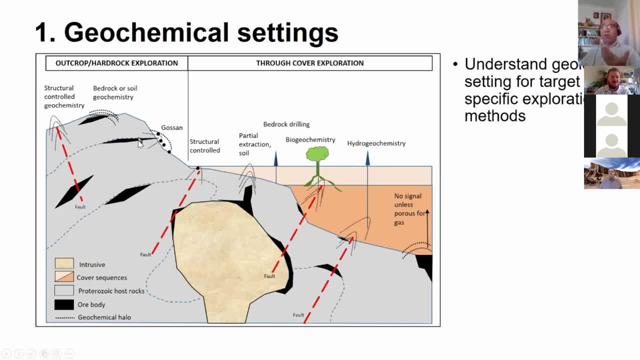 daughter product. you still have a link back to where the original deposit is, as well as the chemical signature is. the third concept is that you know you had the deposit that's deep um inside, but there is a conduit to link the ore deposit to the surface where the sample is taken um by. 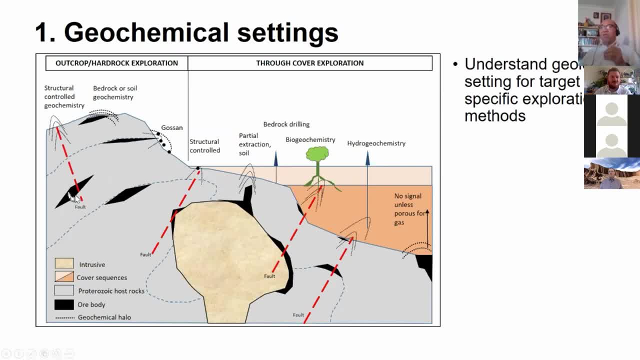 things like fault or, you know, a vent or something like that. and then you have to go back to the, something where the fluids or the material can come to the surface, and you could sample that surface, giving some indication of what the material is at depth, and, like both scenario, you 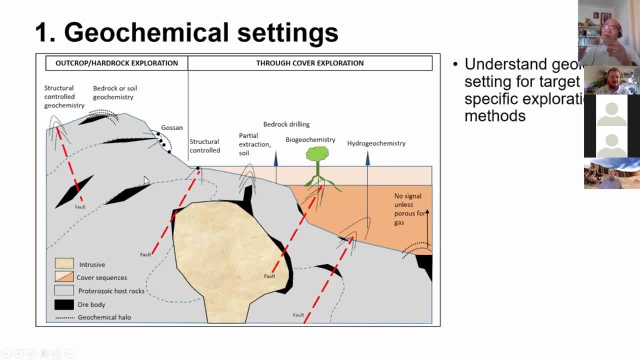 had this last, in a sort of scenario where you had deposits that is deep seated within, it's hidden, that has no signatures to the surface, and these are ones that you know are the biggest challenge, and i believe there's a lot of this in the mind, as in liar, where you need new techniques. 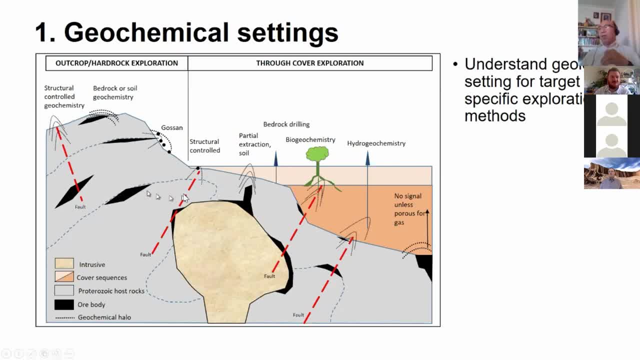 yes, you know um hydrogeochemistry etc. to find this. on the other hand, in the cover sequence itself you have the same scenario, except you had this sedimentary cover that has nothing to do with the ore deposit itself. that acts as a barrier for the chemistry to get right to the surface. 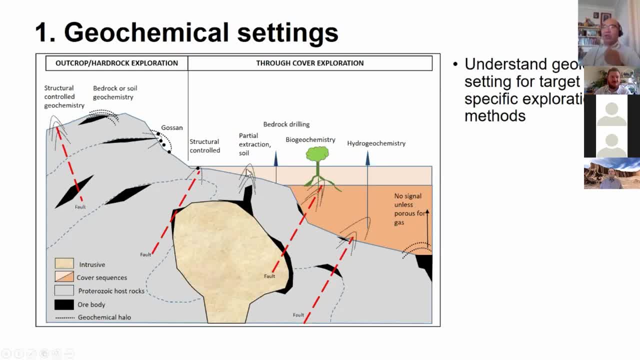 in shallow deposits, the chemistry could still, you know, sort of migrate or diffuse to the surface- and conventional geochemistry might still work- or it forms like a secondary deposit at the unconformable layer, expanding this um footprint, the geochemical footprint, and if it's shallow enough, you can still pick up the signatures. however, in a lot of cases, 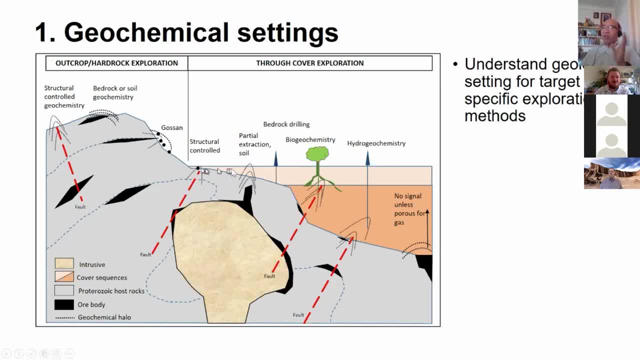 when the sediments gets thicker. this kind of, you know, simple scenario does not exist and a lot of this chemistry are hidden from the surface, although, um, there are a lot of things, like you know, um, the affirmation or dispersion of this chemistry, a long, unconfirmable layer, is what explorers look for, are looking for because it expands the 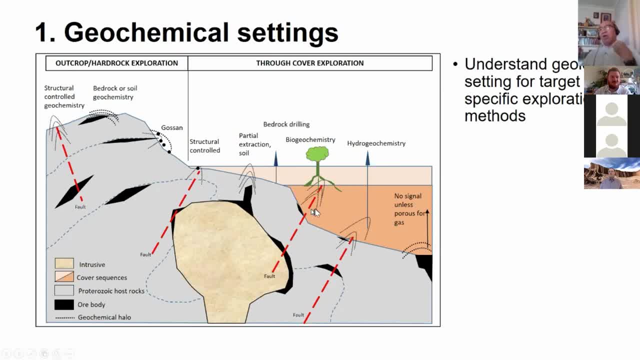 footprint of the chemistry. however, if you get thick cover, it would not come to the surface and therefore you depend on um transfer medium, like, you know, plants, or biochemistry or groundwater, to be able to sort of, you know, um transfer this chemistry right to the surface itself. 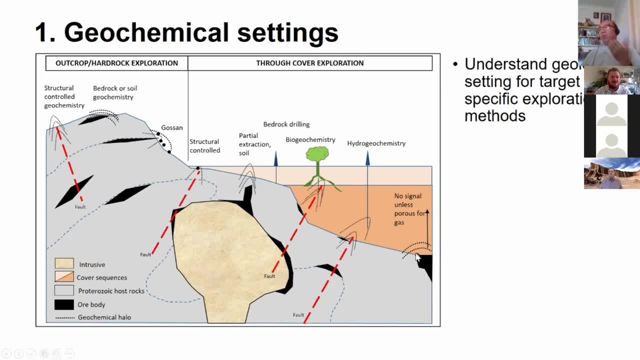 and then you had those hidden deposits. it may be exposed at the um, you know unconfirmed meaty, but it doesn't get to the surface and therefore things like you know porous, you know um, if it's porous enough, salt gas etc. applies. however, you know, in all the scenario for these, 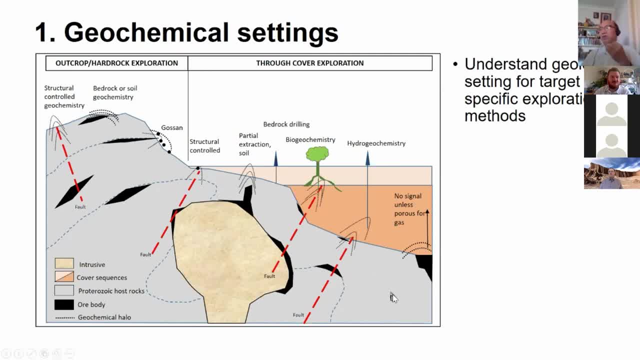 hidden ones. drilling is still in the sort of answer to the discoverer, to the discovery of hidden deposits. so basically, um, in expression chemistry, it's really important to know what geological setting you are in, so that you could choose to write a lot of geological techniques that's suitable for detecting, you know, buried. 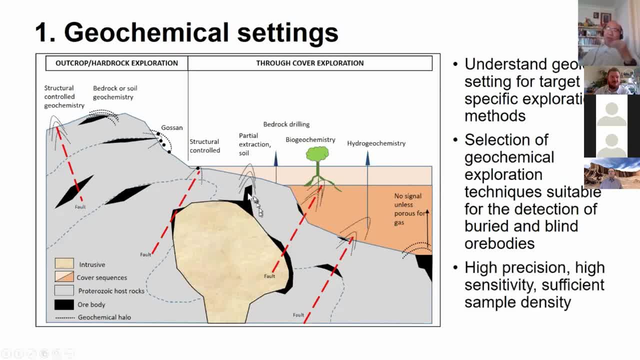 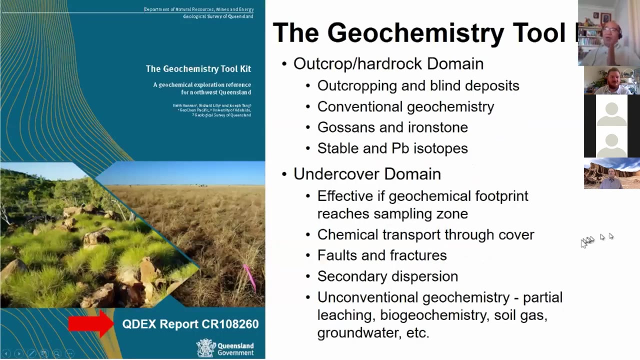 or undercover, or deposit itself, and what's needed, especially in those deep-seated deposits and undercover deposit, it's high precision, high sensitivity and sample that's dense enough, you know, so that you know this signature, this very weak signatures, could still be picked up at surface itself. this leads us to what the geochemical toolkit is. 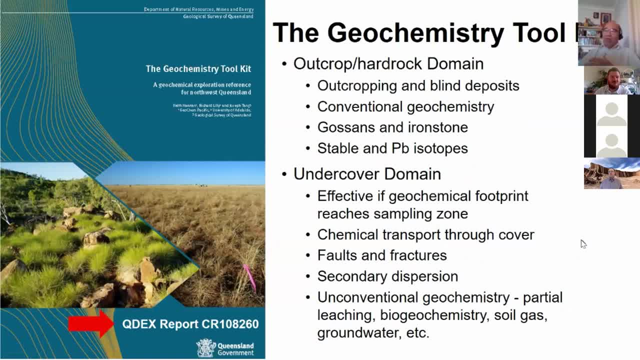 geochemical toolkit summarizes what I've spoken about, you know, in the previous few slides In the geochemical toolkit. it's basically an exploration reference, you know, for the Northwest Queensland. However, it can be expanded throughout Queensland itself because most exploration areas has very 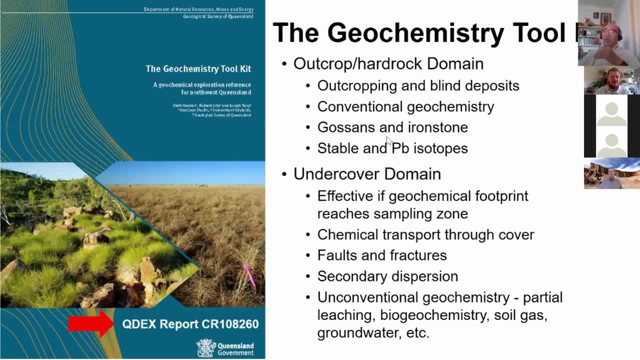 similar setting. The toolkit is divided into two hubs. The first part of this, the first four chapters, talk about the outcrop or the hard rock domain expression. within that, Basically it talks about outcropping, you know, sort of. 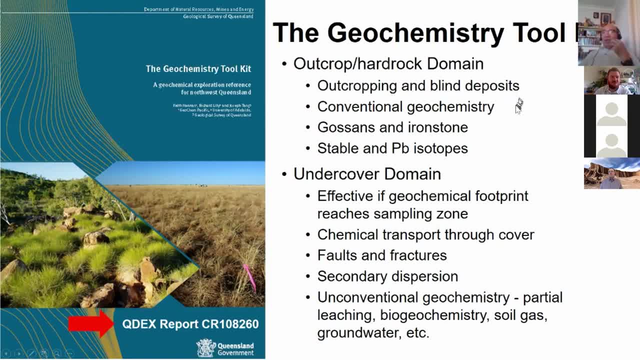 mineralization and blind deposits, And it discusses conventional geochemistry. That's what I talked about early in this talk that you know. you analyze everything to get the best geochemistry to represent all. It also talks about gossams and ironstone, how to differentiate it using filters, And it. 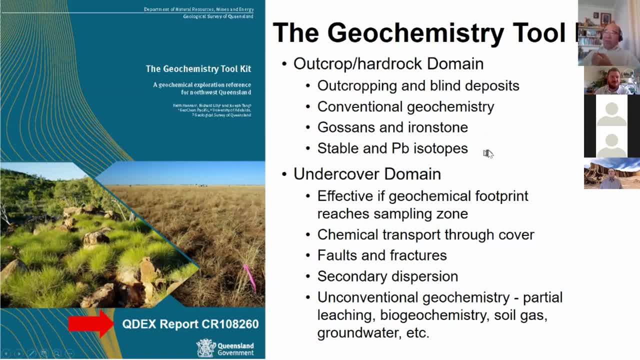 discusses stable and radiogenic isotopes. to determine how you know, sort of you know, to basically model, you know the pathways as well as the potential of mineralization in the area. The second half of it talks about the cover domains. Basically, this only is. 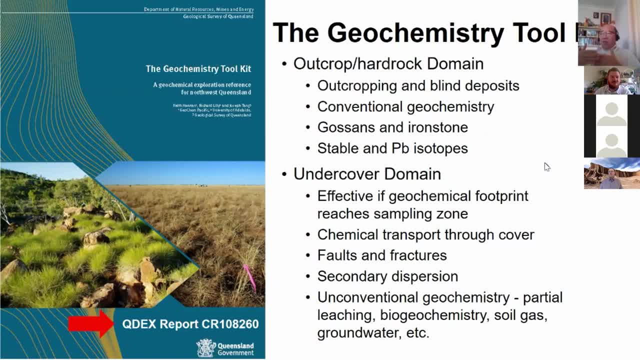 practical if the chemical footprints from the ore reaches the sampling zones And therefore it emphasizes very strongly on the chemical transport mechanism to cover and talks about faults and fractures that access conduits and secondary dispersion, especially at, you know, unconfirmable sort of horizons between the country rock and the sediments above. 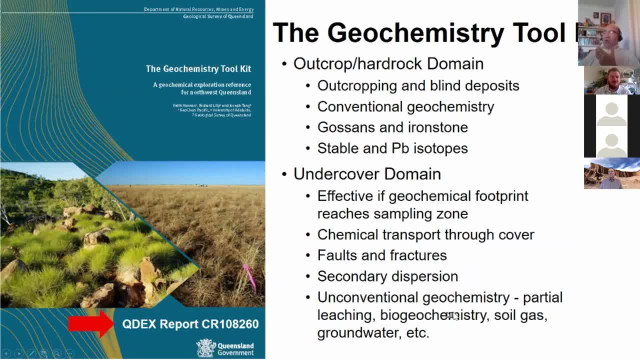 Basically it's very strong on conventional chemistry, discussing, you know, comparing, the different digestions used in some of this example. looking at biochemistry, We tried salt gas and it discussed ground water, you know, sort of in exploration as well. This report is available. 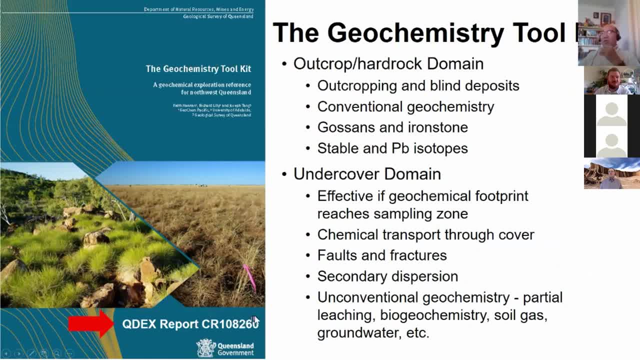 through our QDAC system as report 108-260.. If you download it from QDAC, you also get the all the data that's used to support this modeling, And so I do encourage you to look at the website and, you know, play around with the data And, since it's a published 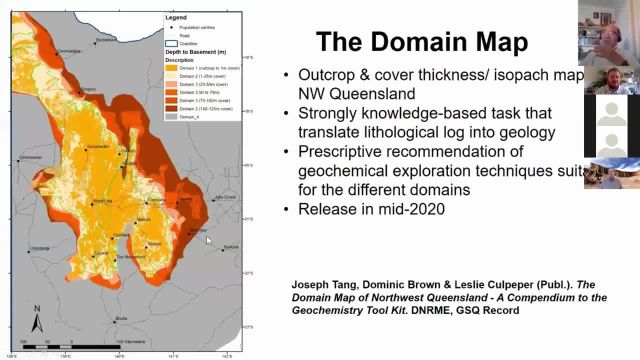 product. I will not go further into this And I'll sort of move on to the next aspect. The next product that GSQ is trying to release is called the Domain Map. Basically, this is, you know, it's an isopack map, you know, of sediment covers around the Mount Isa in Laiezo. 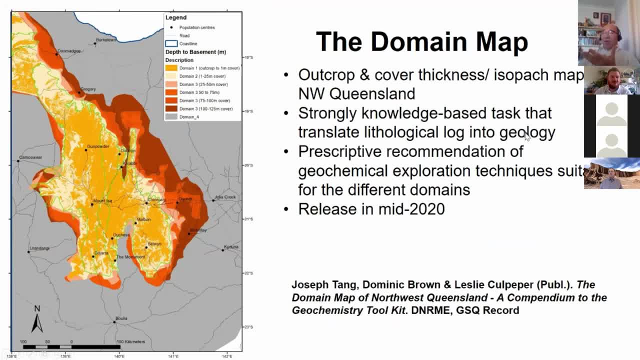 This isopack map is derived from information submitted by company reports through the company reporting system And therefore we basically translate the lithologic logs into geology. The publication also will have a very prescriptive recommendation of the different sample types to use, you know, for these different domains, And therefore it is very similar. 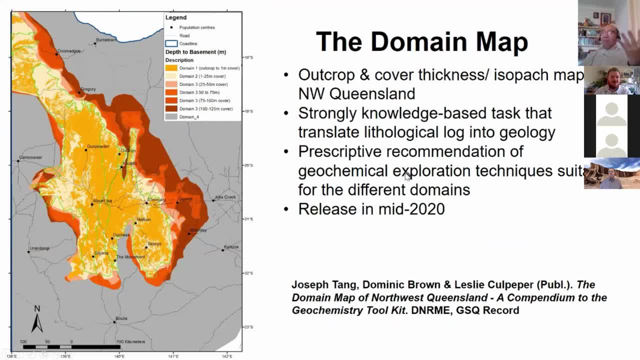 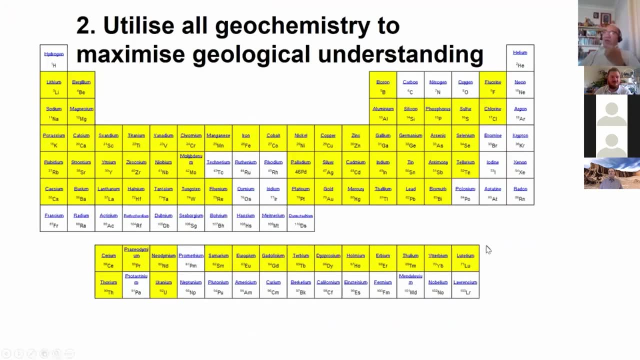 to the toolkit and it's basically complementing each other, And this product, hopefully, will be released by the middle of this year and it should be another sort of you know product that will help you know explorers, especially in the Northwest. The next part of this expression: 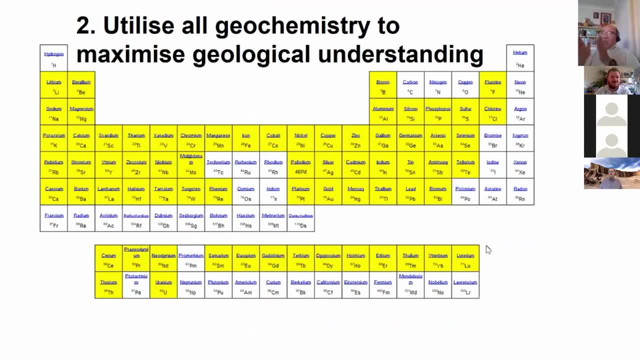 chemistry is, you know, for good success, Successful exploration chemistry- it's really important to understand and use all chemical data to maximize geological understanding. Basically, in most modern analytical- you know- sort of packages, it's able to analyze up to 66 elements. And these are the elements. 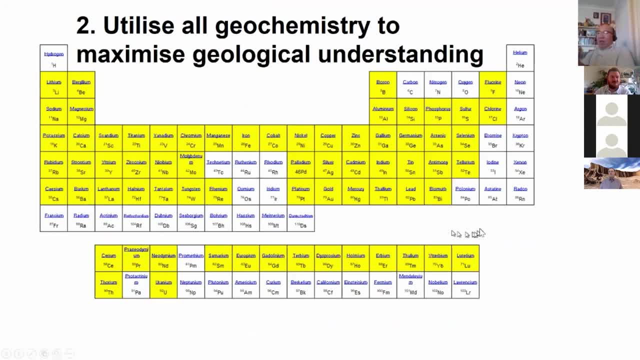 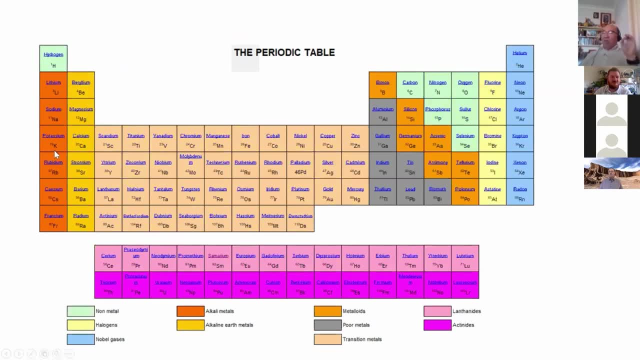 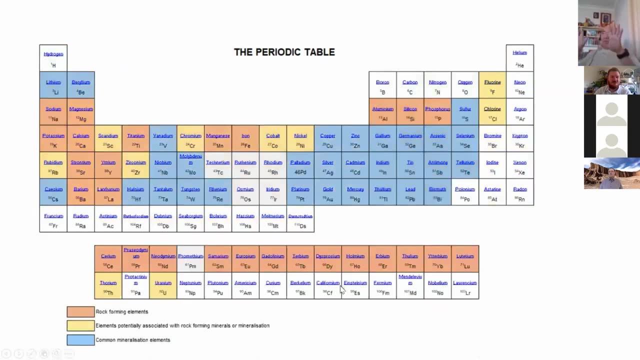 that the labs are able to analyze, you know as the first-pass package, without special techniques. If you look at the different geochemistry, you see that it ranges from alkalic minerals to metalloids to rare earths. However, most of people find it very confusing what. 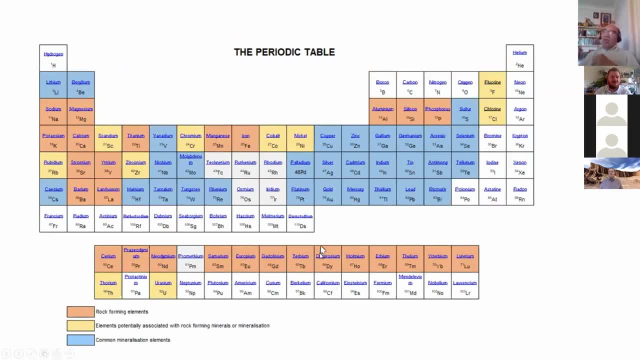 does these different elements represent? Basically, this table indicates the basic control of these chemistries. The ones in beige color basically represent strong lithology control, whereas the one in cream indicates it could be a crossover between rock forming minerals and lithology controls immediately polarization, whereas the colors in blue and 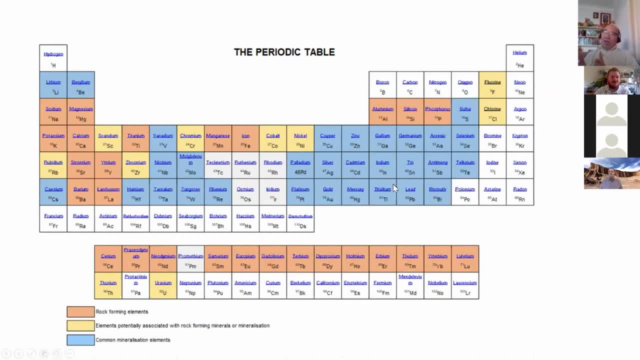 blues are basically all material. So if you've got a high concentration of Tungsten, you are sure that you are in a Tungsten rich ozone already. I've got to get rid of a lot of slides because it's running out of time, but 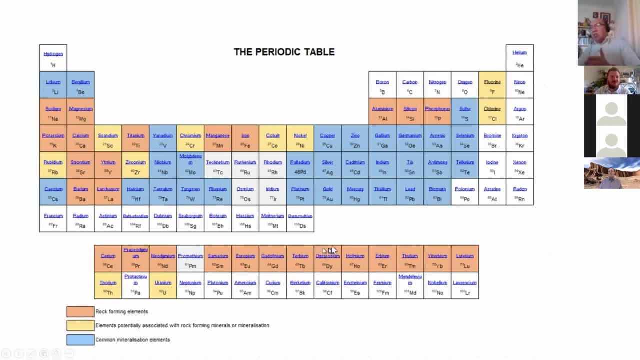 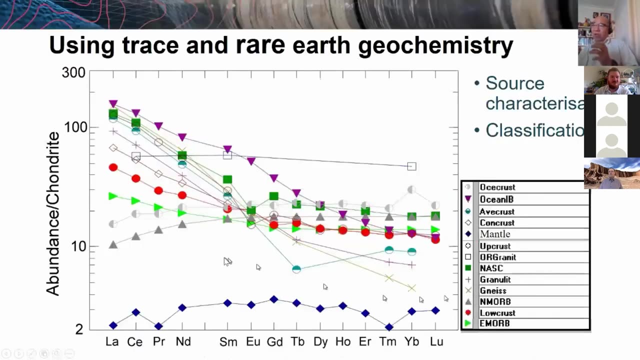 another thing that's important about using chemistry is not to look at single elements but to look at a group of elements and work using multi-elements analysis. that gives you a much better sort of fingerprinting of all systems. Another big question is the trace and ray-earth elements. A lot of people 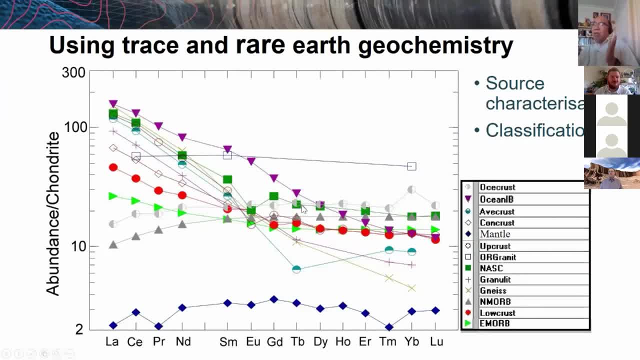 get very confused about this. Basically, they are really powerful elements. The trace elements generally are all material, whereas ray-earth elements will tell you the source, characterization, as well as for classification etc. And therefore I think there are a lot of literature out. 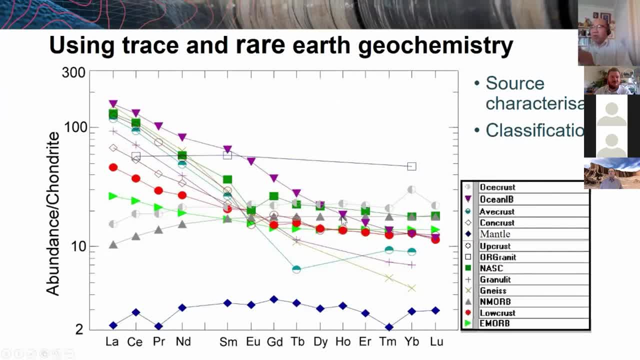 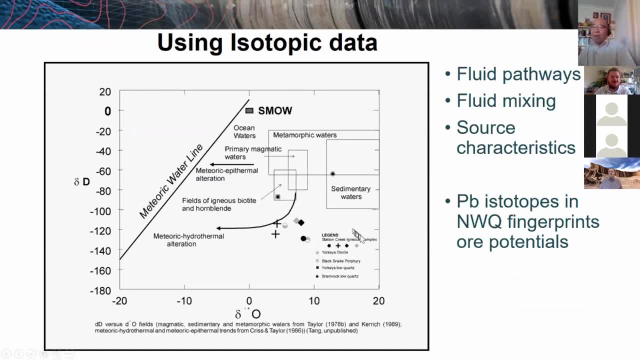 there that you should sort of tap in to find the use of ray-earth geochemistry itself, And also I just put up a sort of diagram of isotope geochemistry. It's a really powerful tool to look at fluid mixtures, fluid sources and 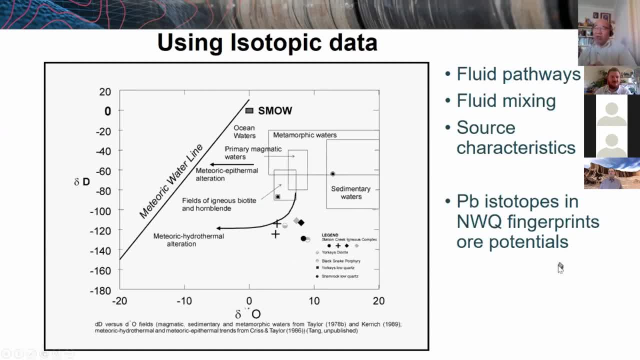 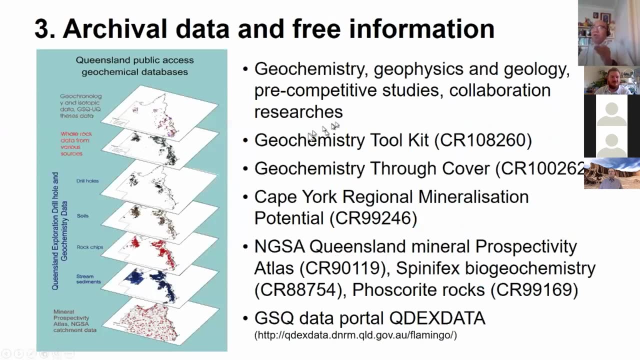 that's for stable isotopes And for radiogenic isotopes, the ones that we mentioned in the toolkit. look at lead isotopes, where it could fingerprint all potential within the monoiso region. Next we'll look at the archival data that's available in Queensland to help. 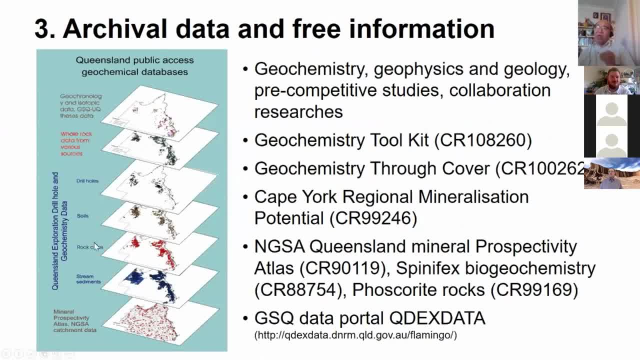 explorers. Basically, what this data does is to de risk exploration in Queensland. There are basically three major packages. The first package that GSQ has sponsored universities to compile their thesis data. however, because of IP rights we can't release it through GSQ. and 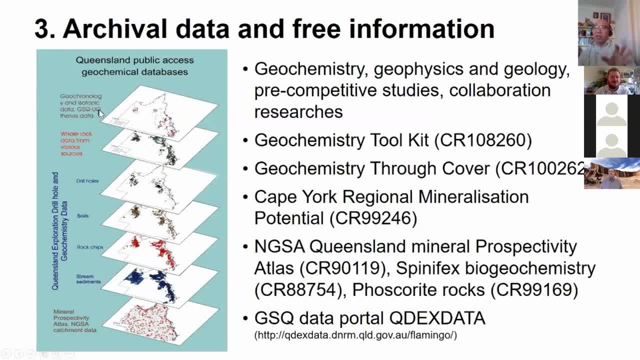 And so most universities have created their own sites to release their data, So we have data from UQ and data from JCU. The second one is Whole Rocks, in which we compile GSQ data, Geoscience, Australia data and UNI data. 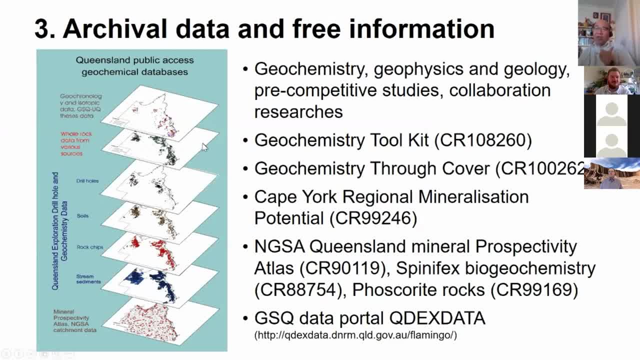 And again, we can't release it openly, but you can write in to us and we can release some of this data to you. The third package- I think Dominic has mentioned this- is Expression Geochemistry. that consists of drill holes, soil, rock chips and stream sediments. 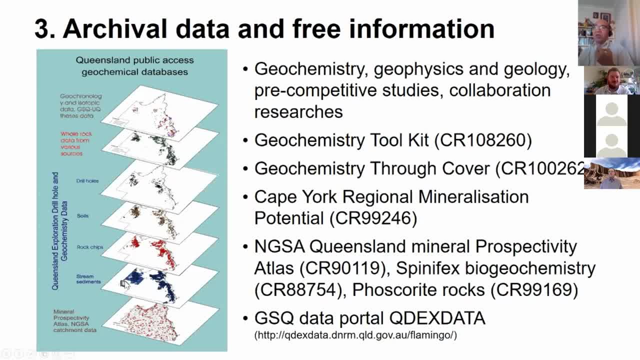 And this is some really very sort of comprehensive data sets and there are. you know that people could use, you know in the exploration And then you know. the last package is the various reports where you had value added. you know knowledge base reports and data to help explorers. 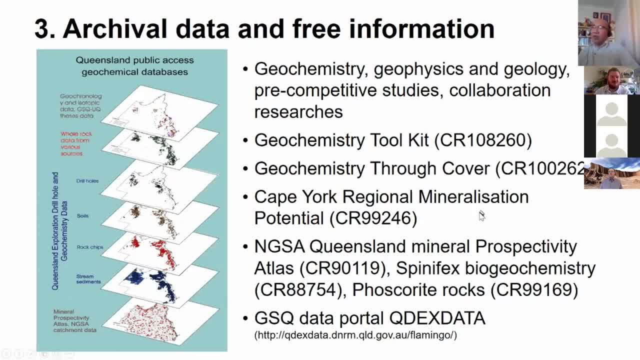 What I've done here is to list some of the sort of projects that's been done by GSQ, or collaborated or funded by GSQ, that you could download. you know, from QDEX. That will help you to de-risk in your exploration within Queensland itself. 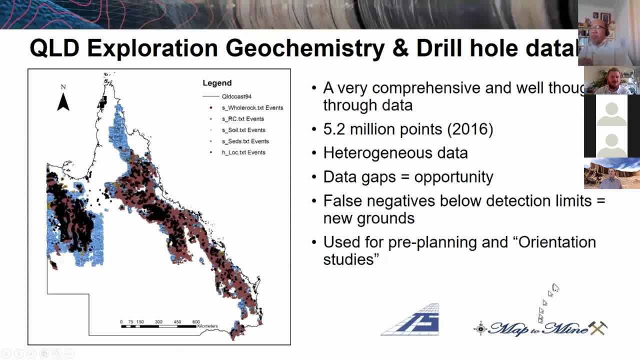 In terms of Expression Geochemistry. this is compiled by TerraSearch and Map2Mind. This is a really good database, I should admit. However, it has a problem that it's really heterogeneous and it's always concentrated in the exposed area of Queensland. 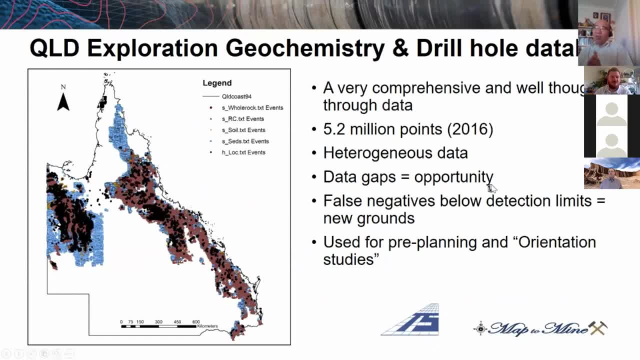 There's a lot of gaps in between the data, and gaps means there's more opportunities in Queensland And there's also a lot of false negative That's below detection. That's below detection limits, which means that there are a lot of area that has been. 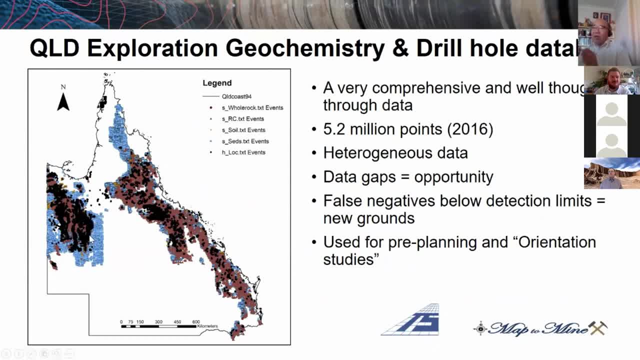 explored, but they are very are analysed using very coarse detection limit, And so lots of these areas, all the geochemistry areas, are probably areas that you could re-examine, and then you know this probably has much more potential in these areas itself. 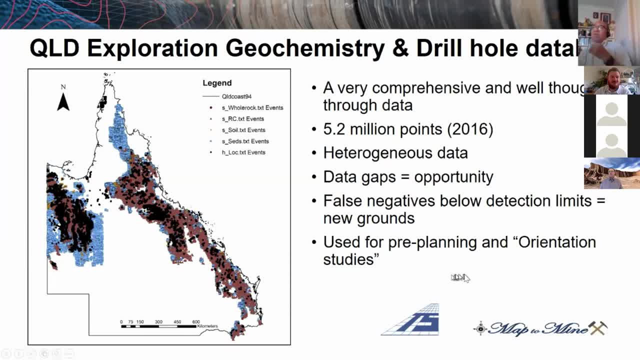 Well, the use of this database is basically for pre-planning And, because of the diversity of data, it could be used as a de-facto orientation study And it's a really powerful tool that I really encourage you to sort of look at it before. 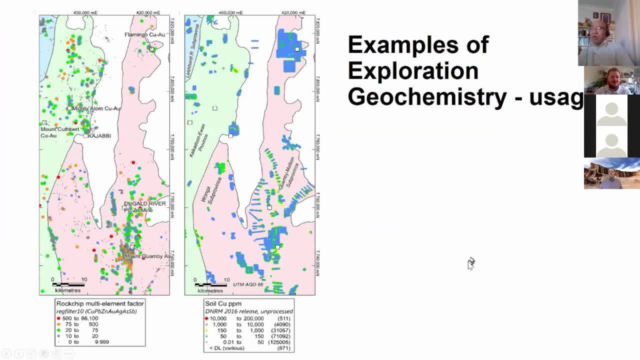 you sort of move on. This is an example of one of the usage. You could use it as a single sort of plot, For example a soil plot of, you know, Mount Asa near the Lansborough graben. or you could 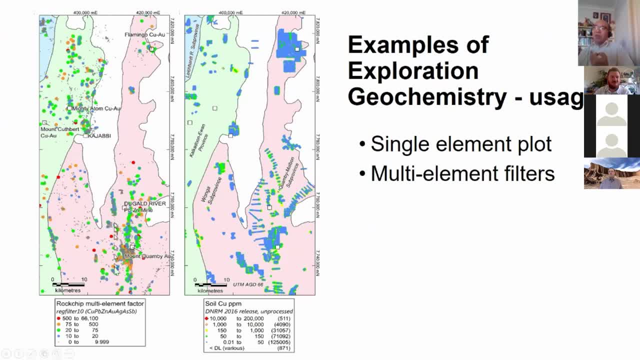 use it as multiple, multiple, multi-elements plots, Like you know. in this case, you could use it as a single sort of plot. You could use it as multiple, multiple, multi-elements plots, Like you know. in this case, you could use it as a single sort of plot. 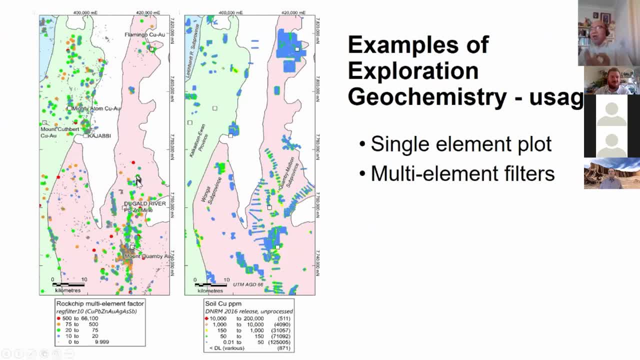 Like you know, in this case you could use it as a single sort of plot. Like you know, in this case you could use it as a single sort of plot And you could use it as a filter to look at it where it highlights a high and low of not. 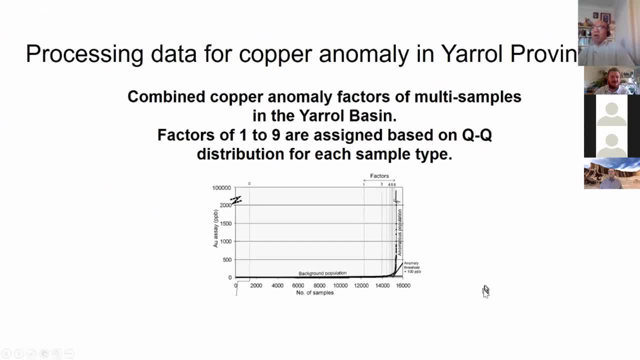 a single element but multiple elements. I mentioned before, it's a really heterogeneous data set with many sample types And this is an example that I've used to process a very heterogeneous sample over the Yarrow Province to look at the prospectivity in that area. 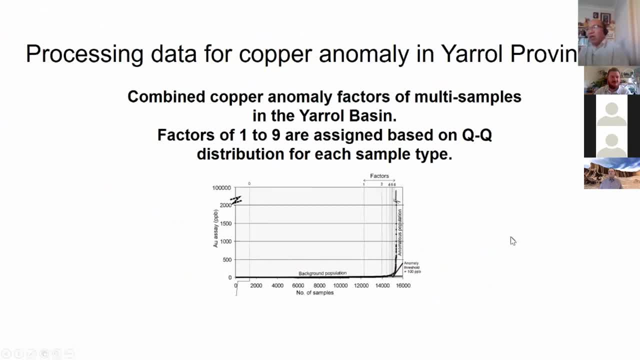 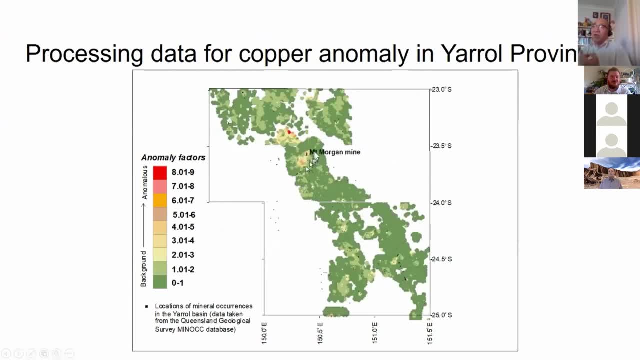 So, basically what I did, I turned those data into factors and combined those factors And this is a plot of the final product, Where it highlights the high and low, For example, this area for copper in it. Is it copper, Yeah? 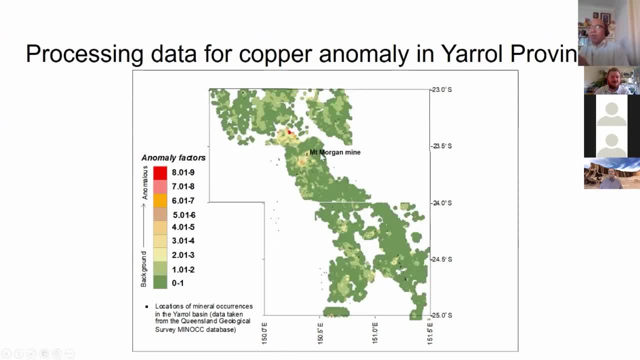 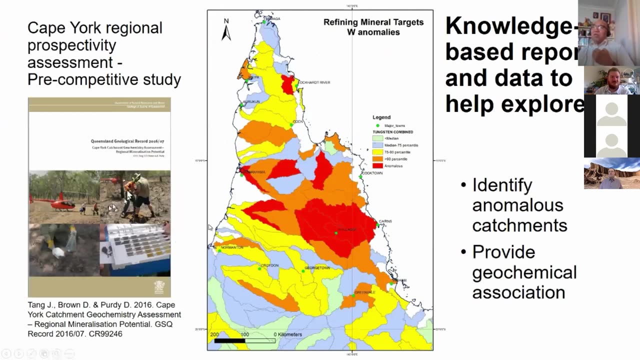 It highlights area of high anomaly around the Mount Morgan area. So this data, it's so diverse and you could use multiple sort of you know techniques to find you know the potential use for that. And the other database that I'm sort of you know that Dominic has mentioned is the Cape. 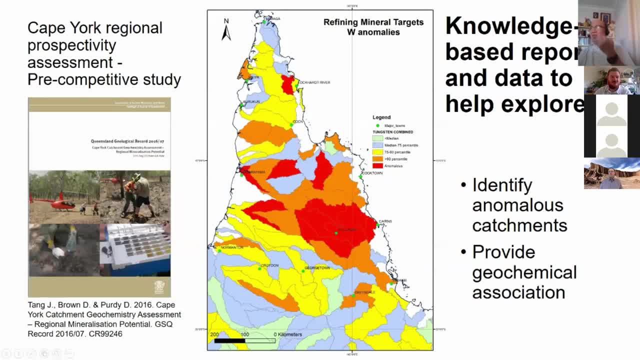 York Prospectivity. And again, this is a knowledge-based data with both knowledge and data incorporated inside it. This first map is the NGSA map for Cape York, for Tansen itself, And it just shows really broad scale anomaly based on that 550 square kilometers catchment. 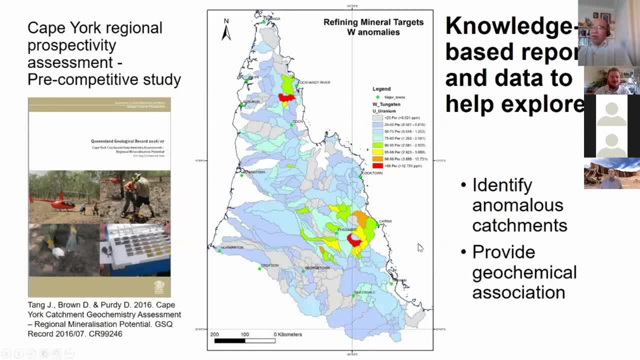 area, But with a more detailed sampling. you know, using this same method on a smaller scale, we could sort of narrow down the Tansen anomaly to very small scale. And this was analyzed. all the sediments were analyzed for 66 elements. 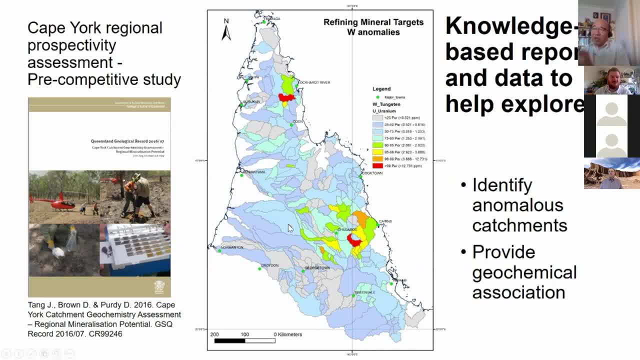 And so you had this multi-elements and also multi sort of catchment database that you could use, you know to, actually as a starting point for exploration. This is also you could see. another sort of example is for Bismuth, for Gold, et cetera. 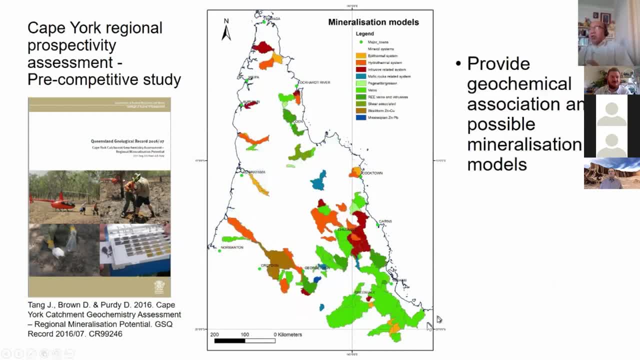 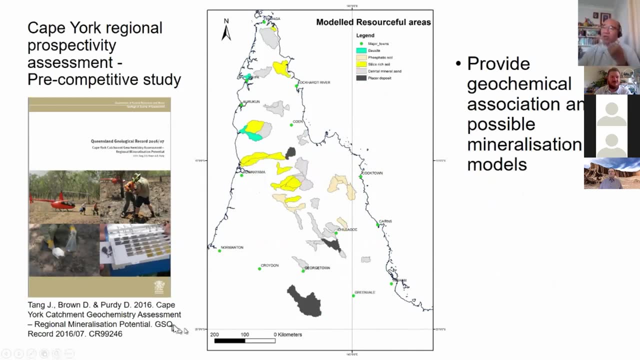 And, being multi-elements, you could combine them as filters or different models to come out with different modeling for the data, And you could also look at the concentration of chemistry to work out the chemical or the resource potential of the region, And so that sort of database- what Phillip and you know has done- has high potential. 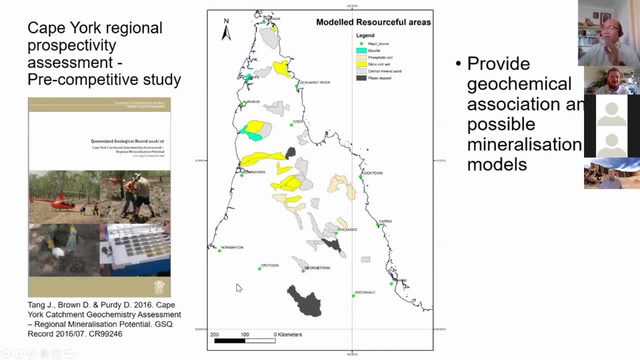 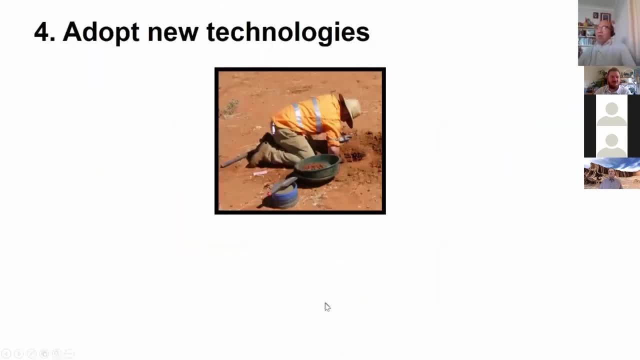 as a starting point for explorers in Queensland, to cut costs, you know, and to go in and target certain areas for mineral potential. And I think you know- I'll just move on really quickly- It's important for explorers to adopt new technologies. 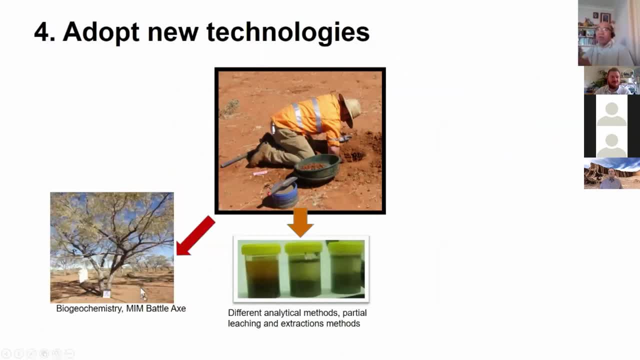 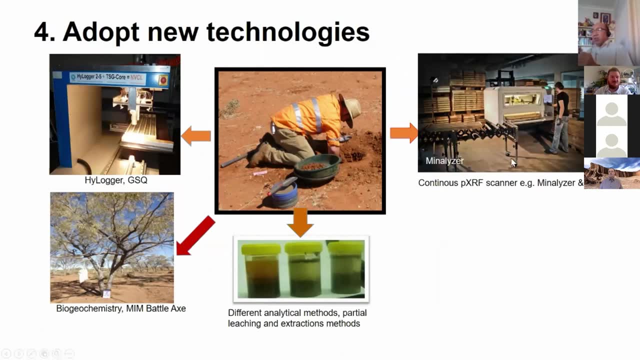 I think I mentioned about the importance of partial extraction, the biochemistry, the high logger where it is like to determine mineralogy and alteration, and mineralizer which does continuous portable XRF scans to determine the chemistry of rock itself, And the other things are portable XRF equipment, hydrochemistry and innovative ways of processing. 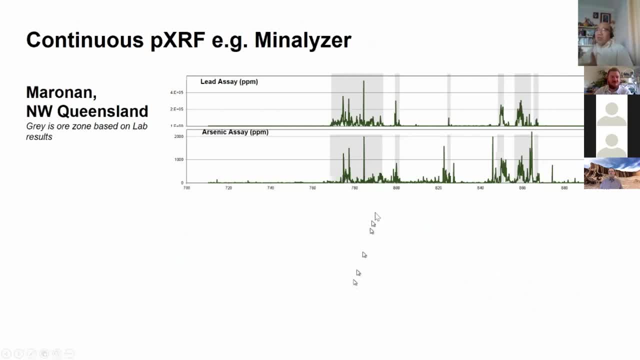 This is an example of results from the continuous XRF. The grays are logging from the geologists and these are pigs actually from the mineralizer- the continuous XRF scanning itself, And if you look at it you could see there are a lot of areas that's missed. but by using 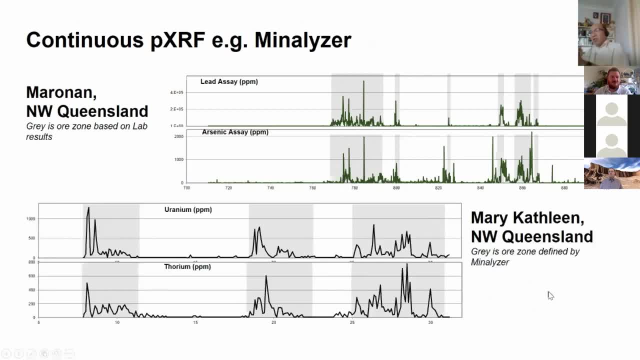 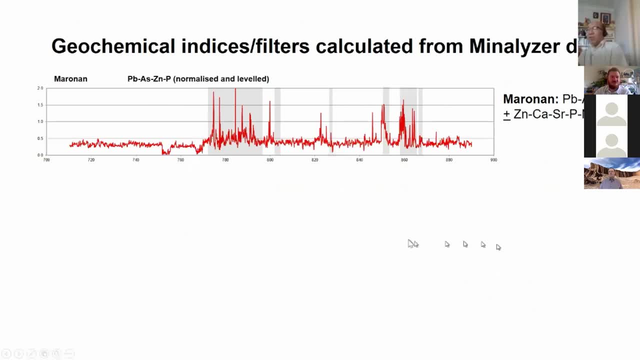 a continuous scan you could sort of pick them up. Similar story with Mary Kay. Again, a lot of these equipments are able to do multi-elements And if you combine multi-elements you can pick up a lot of missed opportunities in that core itself. 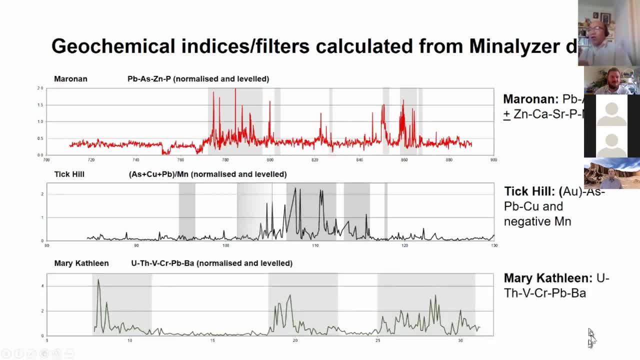 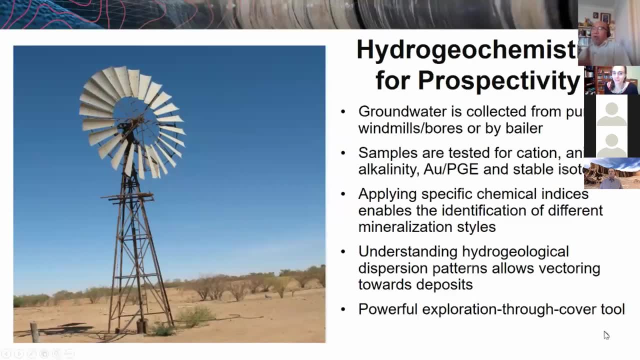 This is for marinin, for tequil and for Mary Kay. You could sort of combine them as filters or indices to determine where the ozone is. And I'll sort of touch briefly. this will be a talk, a future talk of using hydrogeochemistry. 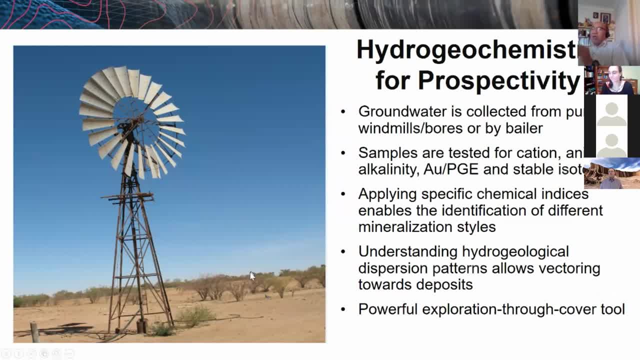 in prospectivity. Basically, the Geological Survey of Queensland has finished a program in the Cloncurry to the Kamilaroi area by taking borehole samples. And you know both from Okay, Okay, We can see. you know we have a bunch of pge and static bores. 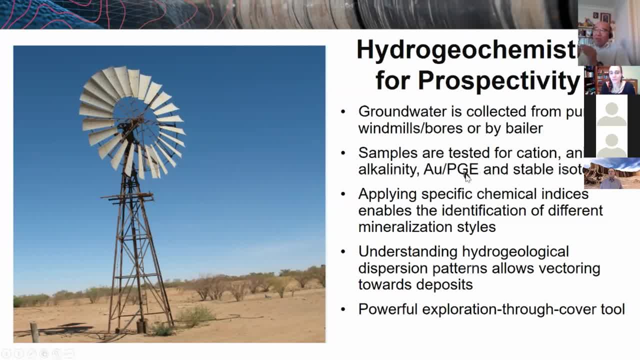 And we look at cation and ions, alkalinity, Golan, PGE and stable isotopes, And then it will be a multi-elements, 60 elements- in a sort of chemistry where we could apply all these indices to understand, you know, the different mineralization styles. 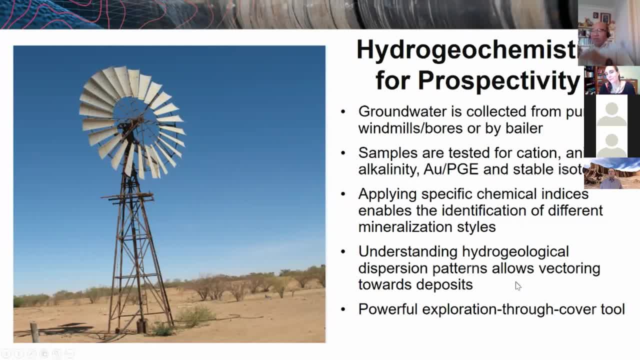 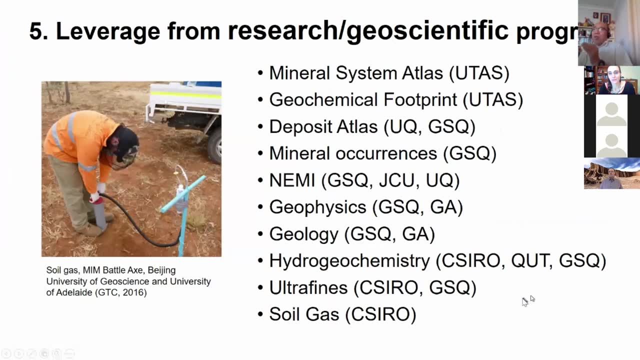 Also, we take you know the depth of the water table, and these information are very useful to vector the water flow And therefore could use the anomaly to predict where potential mineralisation is. Lastly, I stress the importance of leverage from research and geoscientific organisation. I think the Geological Survey,